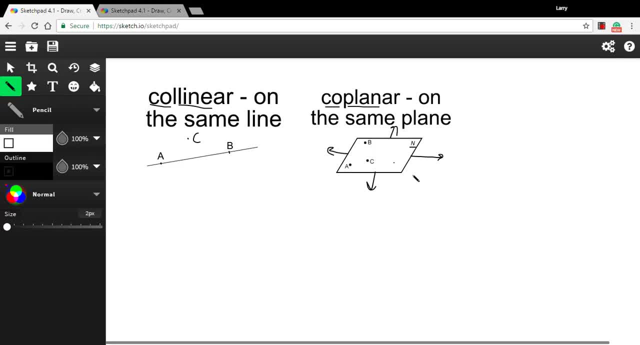 sheet of paper but stretching on forever. If a, b and c are on the surface of that thin sheet of paper, they are coplanar. If point d is hovering above the sheet of paper, then it's not coplanar with a, b and c. Okay, so that's the. 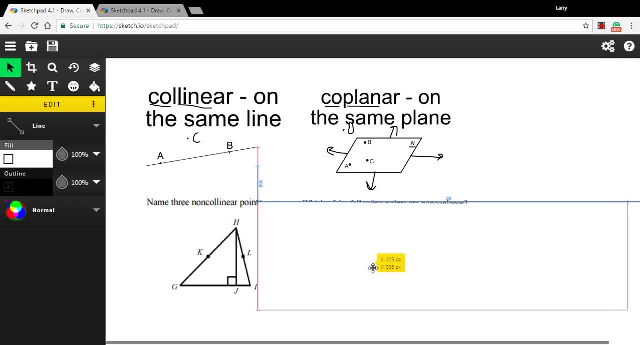 basic definition. Let's look at some problems where you might come across these terms. This one says name three non-collinear points. So non-collinear means not on the same line. Let's look at this problem. Oops, that's filling. Here we go. I could choose l, k and j. Those would be. 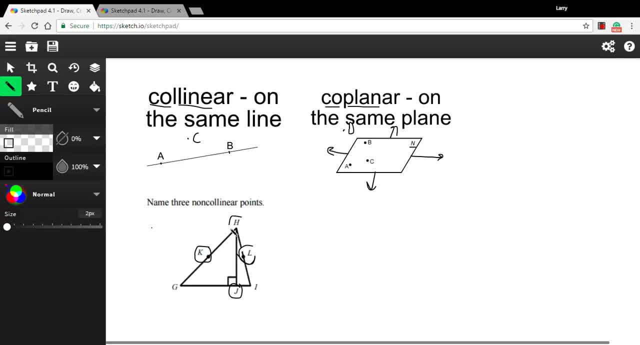 non-collinear. I could even choose l and h and k if I wanted to. Two of those are collinear, but the third one isn't, So altogether the three of them are non-collinear points. So any of those answers. 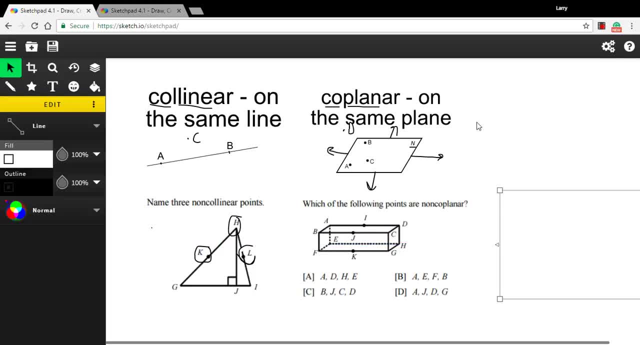 would be acceptable. Let's look at this next problem. This one says which of the following, which of the following points are non-coplanar. And we've got some series of points here. So here's a three-dimensional object, So you kind of have to. 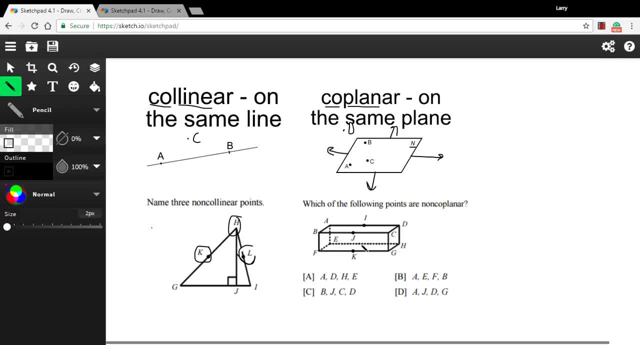 imagine this in your mind's eye: Points that are coplanar. you could set a piece of paper on them and it would touch all the points. So all these points around the top are coplanar, All the points on this side are coplanar, All the points on the bottom are coplanar, et cetera. 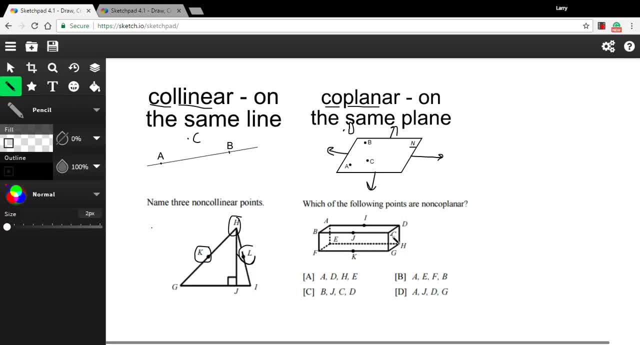 So basically, if you have to fold the piece of paper to make it touch all the points, then they're going to be non-coplanar. So let's see what we've got here. The first one says a, d, h and e. So that's a, d, h and e. Those are all on that back side, So I could push a piece. 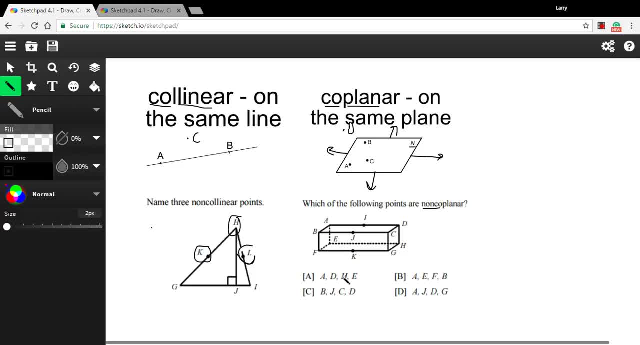 of paper up against that back side and touch them all. So those are coplanar and we're looking for non-coplanar. B says a, e, f and b And that's all the points on this end. right here Again. 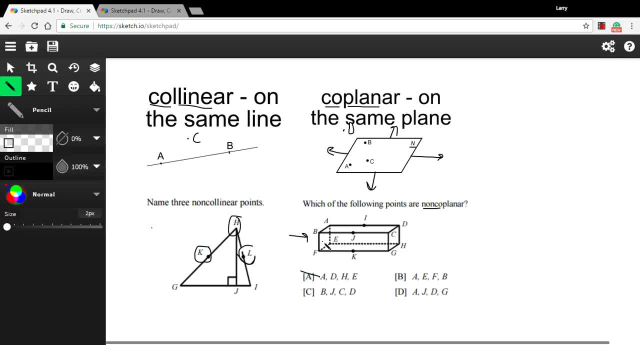 I could snug a piece of paper up against that back side and touch them all. So those are coplanar piece of paper up there without folding it, and touch all four of those points. So it's not that one: B, j, c and d. So here's b, j, c, Oh, and d is over here. So b, j and c are along the front. 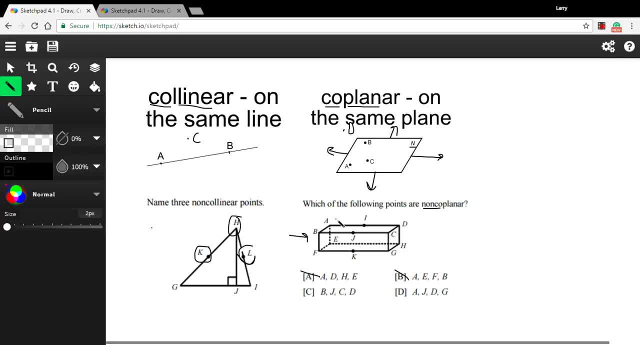 D is in the back. Aha, but we could put a piece of paper on the top and touch all those points. So those would be coplanar two. Hopefully d is the right answer here- A, j, d and g. So 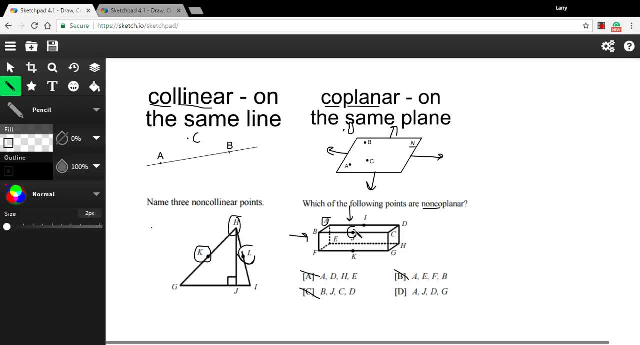 here's a, here's j. Those two are on the top. Now d and g. D is also on the top, Aha, but g is on the bottom. So there's no way I could touch all of those points without having to fold that. 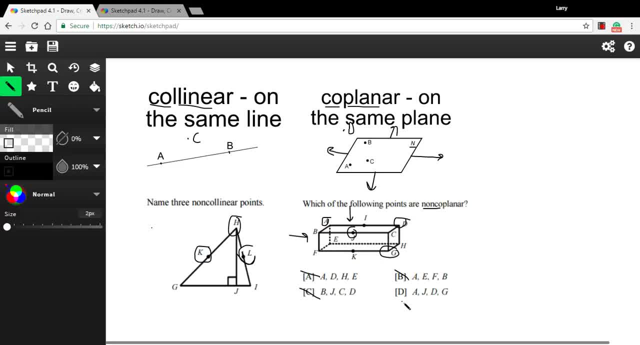 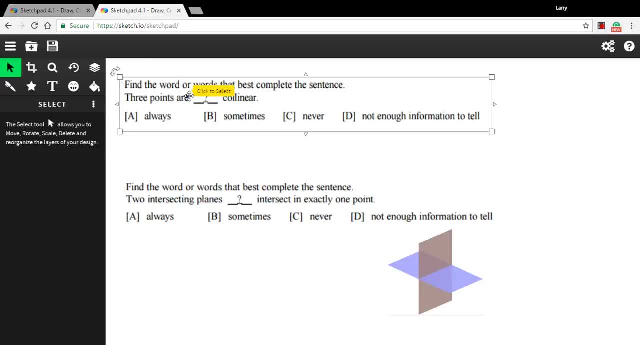 plane. So these are non-coplanar points. Let's look at a couple more problems. This one says: find the word or words that best complete the sentence and it says three points are blank, collinear. and is it always collinear? sometimes never or not enough information to tell. well, collinear means. 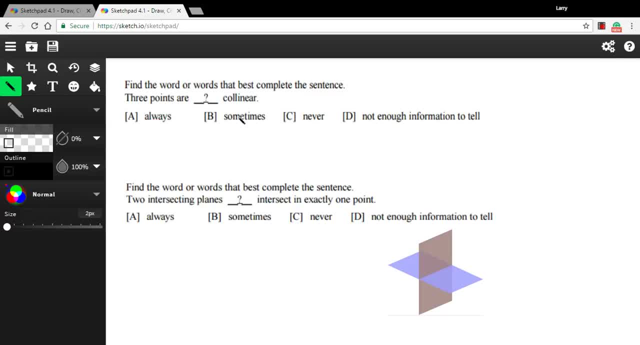 that they're all in the same line. let me just choose the pencil here. so our three points always on the same line? well, I don't think so, because I could have two points on the same line and a third point up here, and you know these might. 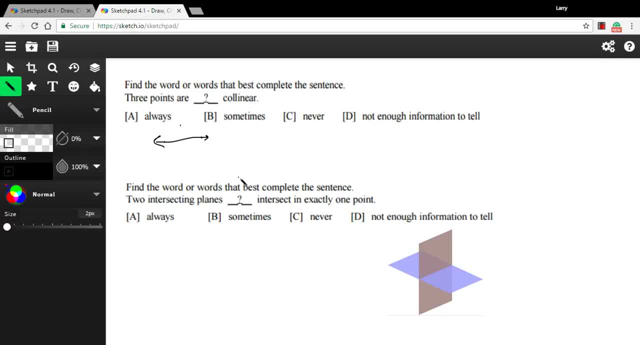 be collinear, but the third one wouldn't be, although I suppose they could be right. I could have a line and have one, two, three points all in a row on line, so they could be. so it's not going to be never and it's not going to be always so. 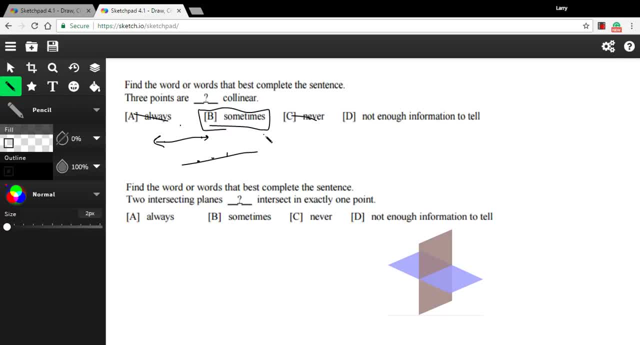 in this case, our best choice is sometimes: all right, let's look at one more. it says: find the word or words that best complete the sentence to intersecting planes always, sometimes or never, always, sometimes or never, always, sometimes or never intersect at exactly one point. well, this might be a little hard to visualize.